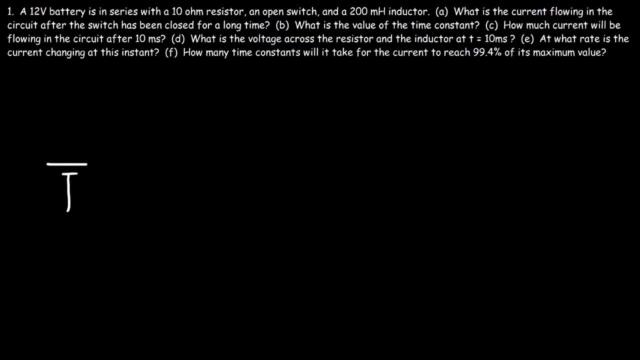 inductor. So let's draw a circuit. So here's the battery and then here is the open switch with the resistor and the inductor. Now what we have is a 12-volt battery and this is a 10-ohm resistor and a 200 milliHenry. 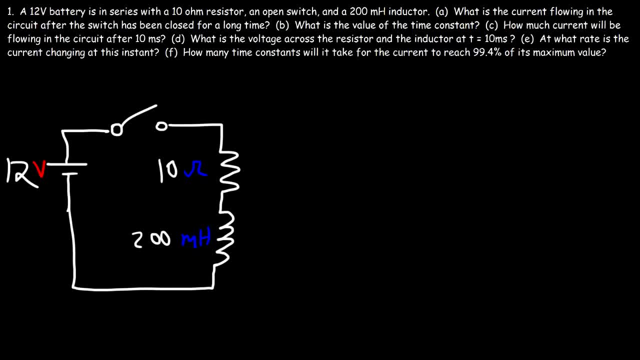 inductor. What is the current flowing in the circuit after the switch has been closed for a long time? So at T is equal to infinity. the current is going to be at a maximum once we close the switch, And so that maximum current is simply the voltage of the battery divided by the resistance. 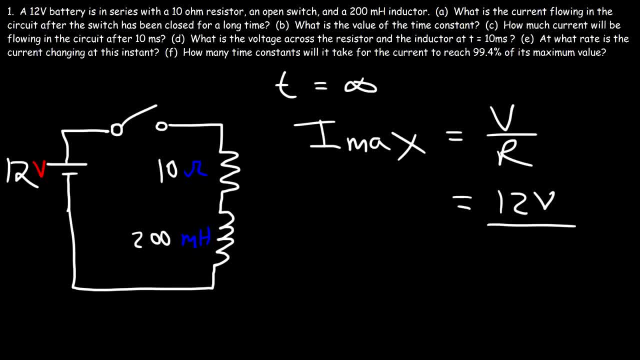 of the circuit. So it's going to be 12 volts divided by 10 ohms, which is 1.2 amps. So the maximum current, which I'm going to call I0, that's 1.2 amps. And so that's the answer for part A. 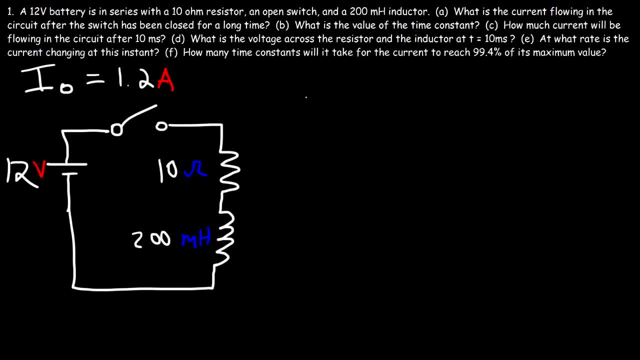 Part B. What is the value? What is the value of the time constant? The time constant is represented by the symbol tau And to calculate it it's equal to the inductance divided by the resistance. So the inductance is 200 milliHenrys, or 200 times 10 to the minus 3 Henrys. 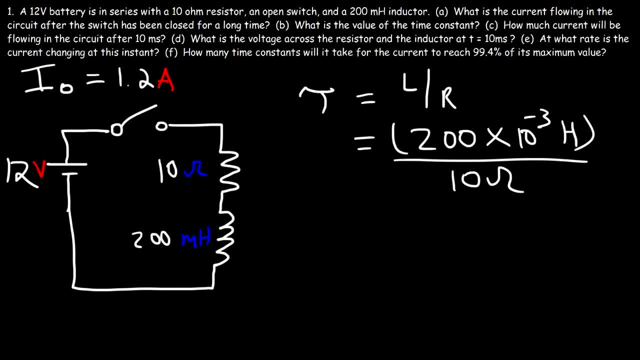 And the resistance is simply 10.. So the time constant is 0.02 seconds, Which I'm just going to rewrite this here. And so that's it for part B. Now part C: How much current will be flowing in the circuit after 10 milliseconds? 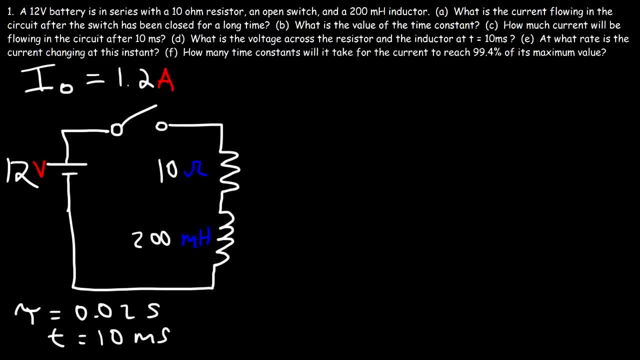 So after a time period of 10 milliseconds, what is the current Now one second is 1,000 milliseconds. So to convert 10 milliseconds to seconds, divide it by 1,000.. So 10 divided by 1,000.. 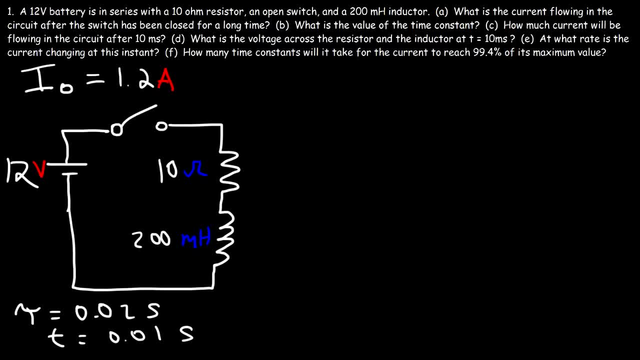 It's 0.01 seconds. So now, how can we use this information to calculate the current? When the switch is closed, the current is going to increase from 0 to 1.2.. And so we're going to have a graph that looks like this: 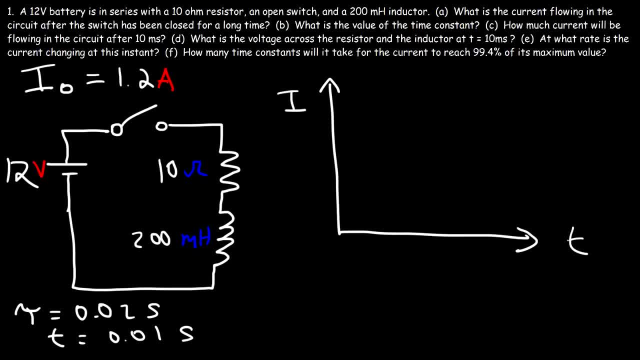 So this is the current on the y-axis, On the x-axis is the time And this is the maximum current. So that's 1.2 amps, And so it's going to start from 0. And gradually increase to its maximum value. 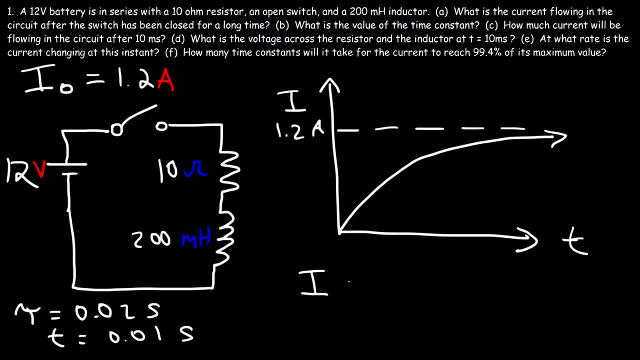 And so that graph is represented by this formula. So the current is going to be the maximum current times, 1 minus e raised to negative t divided by tau. So in this example the maximum current is 1.2 amps. The time is 0.01 seconds. 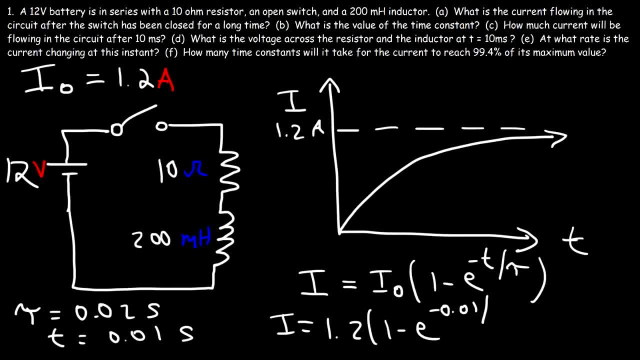 And the time constant is 0.02 seconds. So this is going to be the maximum current times: 1 minus e raised to negative t divided by 0.02 seconds. So go ahead and type that in exactly the way you see it. 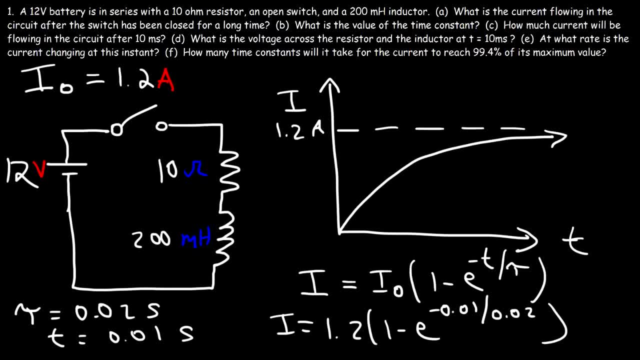 So the current at 0.01 seconds is going to be 0.472.. So the current at 0.01 seconds is going to be 0.472.. So the current at 0.01 seconds is going to be 0.044 amps. 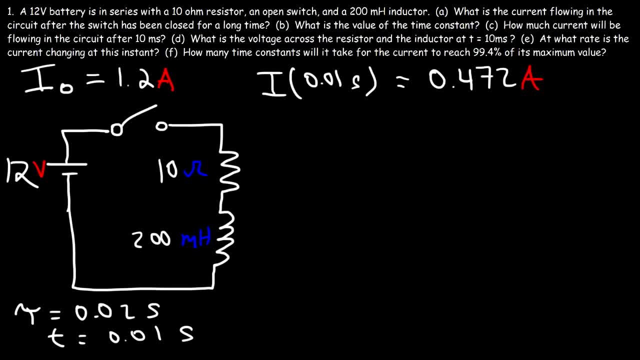 Now there's another equation that you need to know when dealing with inductors. You don't need it for this problem, but this is just some extra information. Let's say, if the switch is closed and then you open the switch, You need to know what happens when the inductor releases the energy that's stored in a magnetic field. 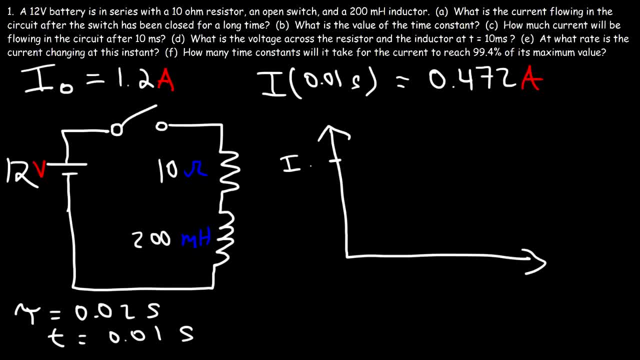 So when it releases the energy, you need to know what happens. when the inductor releases the energy that's stored in a magnetic field energy, the current is going to start from its maximum value and it's going to decrease like this, and the equation that corresponds to that graph is this: 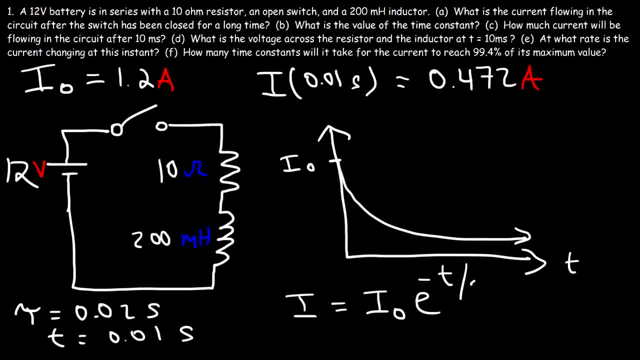 equation. so you need this equation if the current is decreasing, if the energy is being released by the inductor to the circuit. and for the other equation, let's say if energy is going into the inductor, if the current is increasing. that is this situation. it's going to be. I is equal to I 0, 1 minus e negative T over. 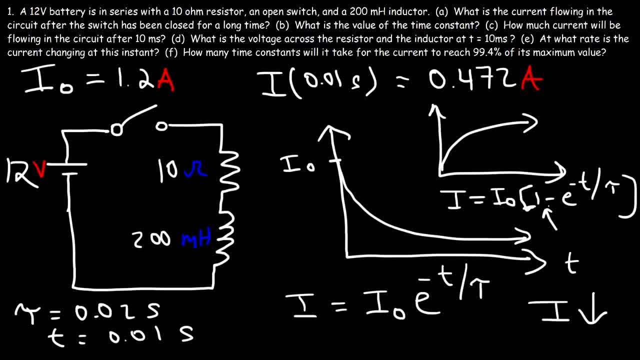 tau. so the difference is the one that's when the current is increasing, but if it's decreasing, just that one is not going to be there. so those are some equations that you want to use for this type of a problem. now let's move on to Part D. what is the voltage across the resistor and the 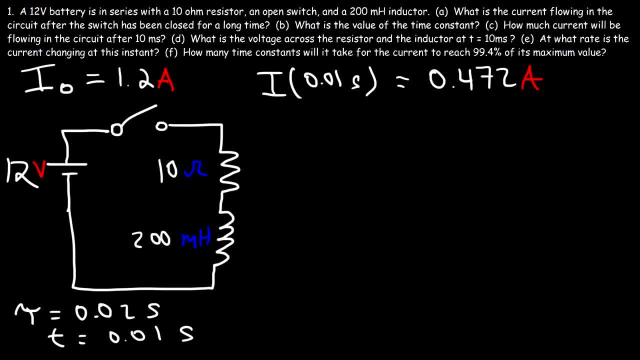 inductor at T equals 10 milliseconds. so at 10 milliseconds we have this current. so the voltage across the resistor- it's just going to be the current that flows through the resistor- times the resistance. so the current at this instant is 0.472 amps and resistance is 10 ohms. 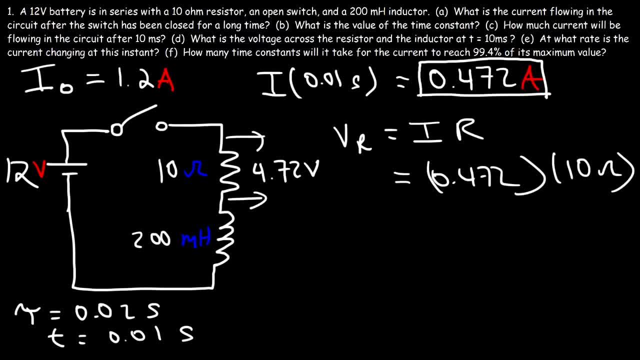 so then that's going to be a voltage of 4.72 volts. now, to calculate the voltage across the inductor, we need to realize that the voltage drops must be equal to the voltage of the battery. so it's going to be 12 minus 4.72. so the voltage 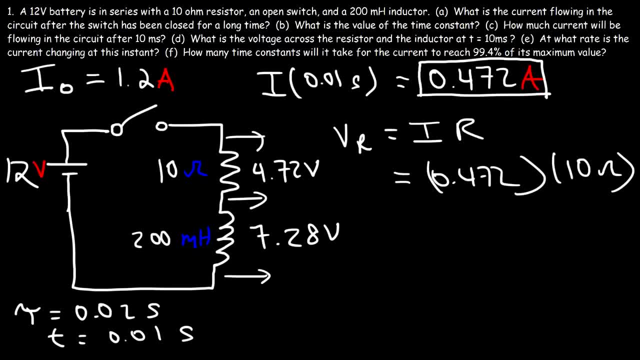 across the inductor is 7.28 volts. now it's important to understand that this voltage is positive because that battery delivers energy to the circuit and these they're negative because, as the current increases, they consume energy from the circuit so they cause the voltage drop. so VL is negative, 7.28 volts, technically speaking. now Part E at 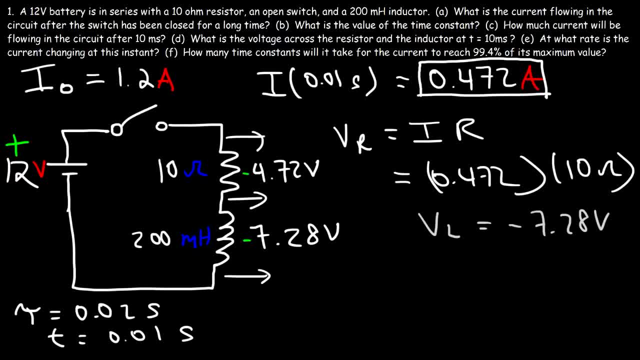 what rate is the current changing at this instant? so the EMF across the resistor and the inductor is equal to the inductance. it's negative L times the change in current divided by the change in time. in some textbooks you'll see it as di over dt and for the most part di over dt is approximately the same as. 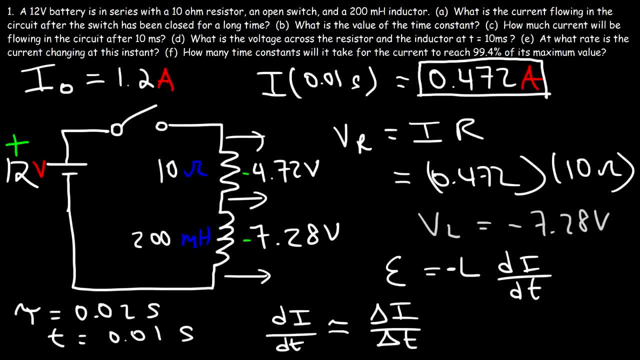 Delta I over Delta T. it's the change in current per change in time. now the EMF induced by the inductor is this value. so that's negative 7.28 and that's equal to negative L, which is 200 times 10 to the minus 3 times di dt, so negative 7.28. 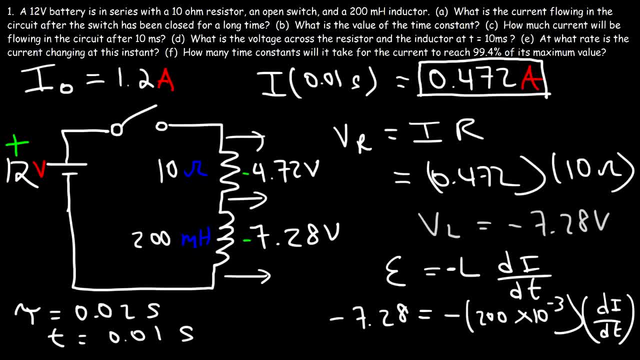 divided by negative, 200 times 10 to the minus 3, that's equal to this number. but let me make some space. first it's positive: 36.4 amps per second. so that's the rate at which the current is increasing per second. now we know should be positive because we're dealing with 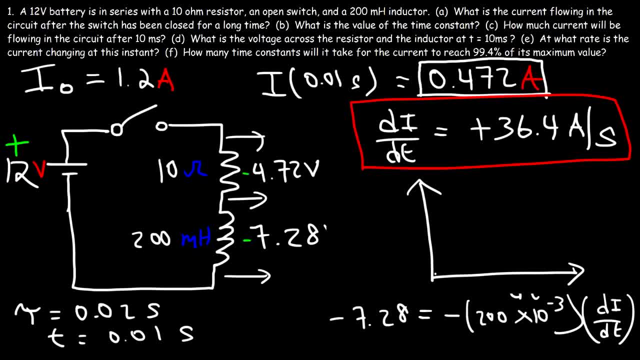 this situation: when the switch closes, the current is going to increase from 0 to 1.2, so therefore the current is increasing. di. dt should be positive, which means the voltage across the inductor has to be negative, which fits well with this equation. so it's important to 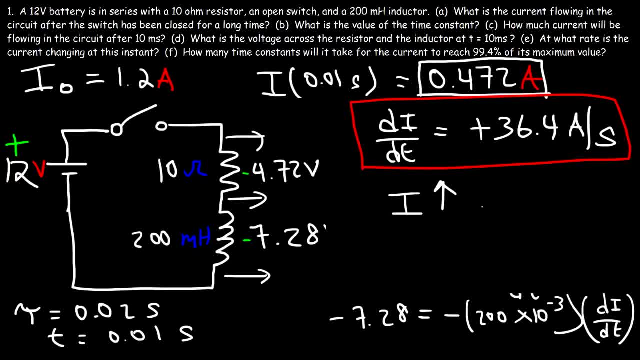 understand that as the current in the circuit increases the inductor, it stores energy, so it's absorbing energy from the circuit and that energy is used to build up the magnetic field that's inside the inductor. so the EMF generated by the inductor is negative, that's the induced EMF. if the current is decreasing the 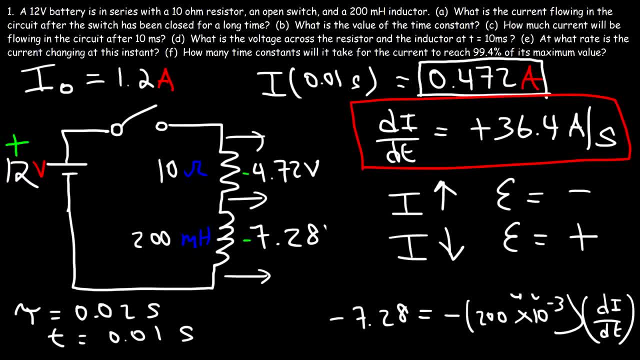 induced EMF will be positive. so you're going to have a collapsing magnetic field and the energy that's stored in that magnetic field is being transferred back to the circuit. so if you increase the current in the circuit, the inductor is going to try to oppose that increase in current and it's going to absorb. 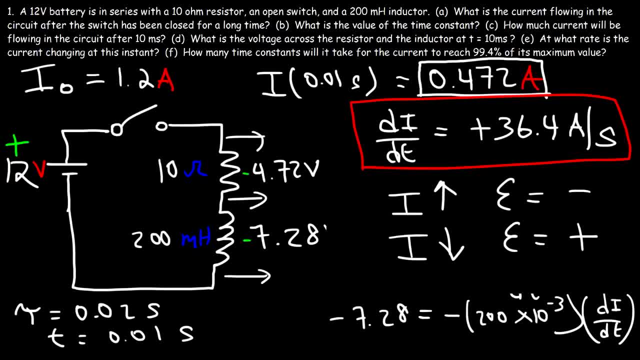 energy, causing the current to increase slowly rather than rapidly. now, if the current decreases, the inductor is going to use its stored energy and it's going to release it into the circuit in order to maintain the current and, as you can see, when the current decreases, the EMF is positive. the inductor is trying to 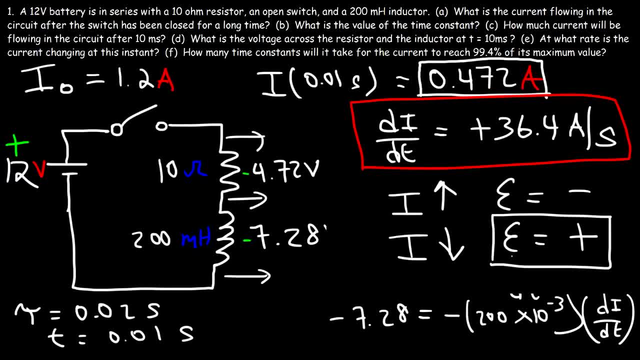 support the decrease in current. so those are some things to know. so if the current is increasing, the voltage across the inductor is a voltage drop, just like the resistor. the resistor absorbs energy from the circuit, but if the current is decreasing, the inductor will be able to support the energy from the circuit and 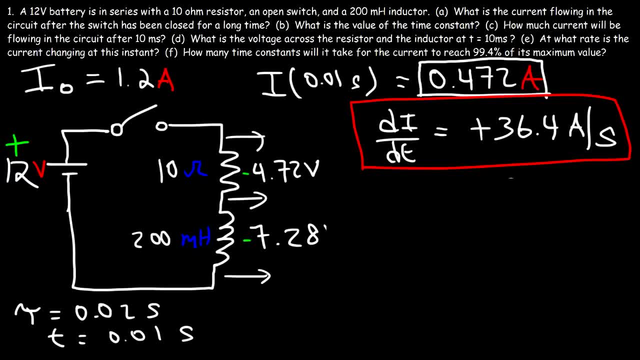 will be basically what's the word I'm looking for. it's going to act like a battery. it's like a voltage boost or voltage lift. it's going to increase the energy of the circuit if the currents decreasing. now let's move on to the last part of this problem. how many time constants will it take for the current? 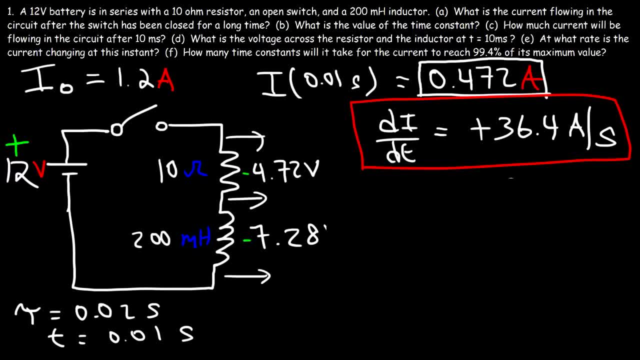 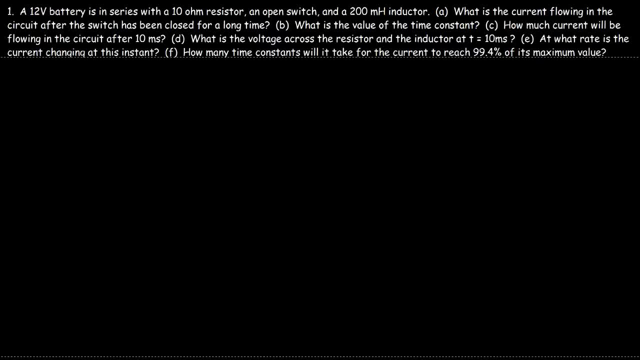 to reach 99.4 percent of its maximum value. so keep in mind tau is .02 seconds. so first let's start with this equation. so the current is equal to the maximum current times, 1 minus e raised to the negative T divided by tau. so let's rearrange the equation and solve for T. 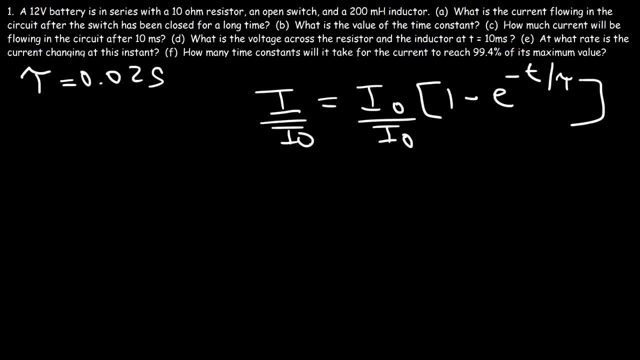 so first let's divide both sides by i0, the maximum current. so we have i divided by i0 and that's equal to 1 minus e raised to the negative T over tau. so what I'm going to do now is I'm going to take this term. 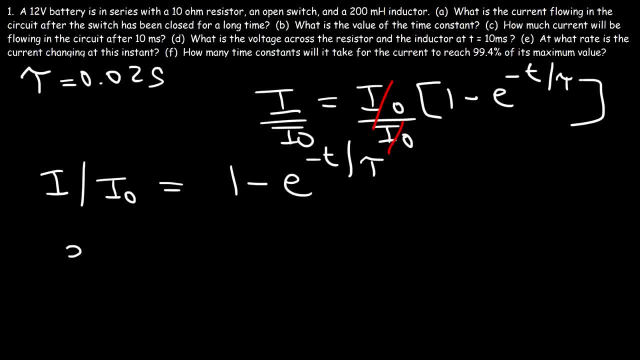 move it to this side where it's going to be positive e. and then we're going to take this term- move it to that side where it's going to be negative. so I'm going to have 1 minus i over i0. so now I'm going to take the natural log of both. 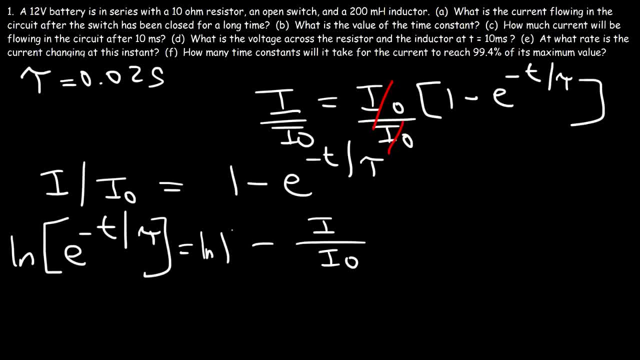 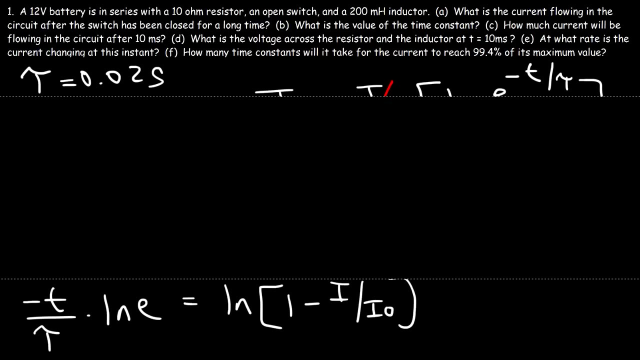 sides. a property of logs allows you to take the exponent and move it to the front. so now what I have is negative T divided by tau times the natural log of e, and so that's equal to ln 1 minus i over i0. so at this point, 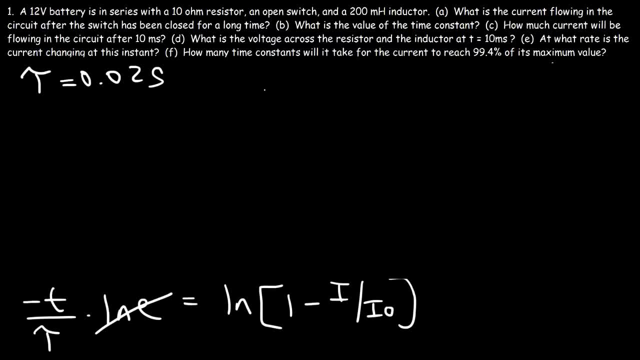 we can get rid of ln e. ln e is equal to 1, so we have negative T. divided by tau, that's equal to ln 1 minus i over i0. so now I'm going to multiply both sides by tau, and so these will cancel. 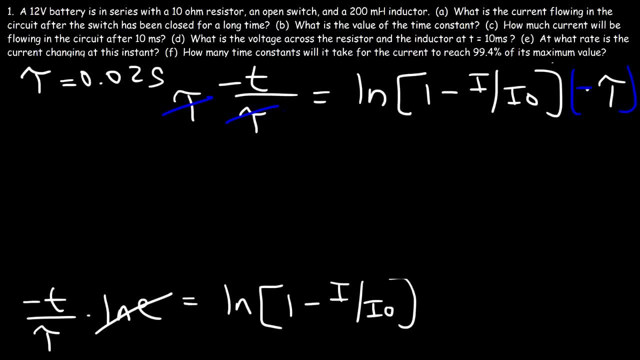 I'm going to multiply both sides by negative T, so I can get rid of the negative sign as well. so T is equal to tau. that is, negative tau times the natural log of 1 minus i over i0. so now let's finish it. so I want to. 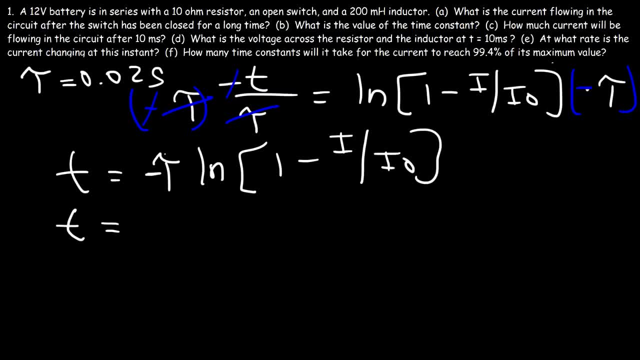 get the number of time constants, so I want to get T in terms of tau, so I'm not going to replace tau with 0.02 seconds right now. now we want the current to reach 99.4% of its maximum value. the maximum value is 100%, so I'm just going. 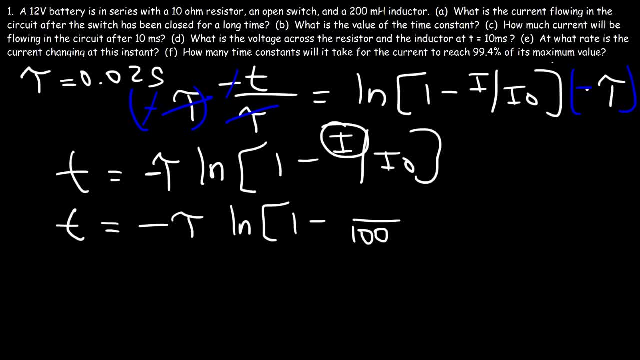 to replace i0 with 100, and I'm going to replace this with 99.4%, which is what we want to reach. so 99.4 divided by 100 is 0.994. so ln 1 minus 0.994, that's equal. 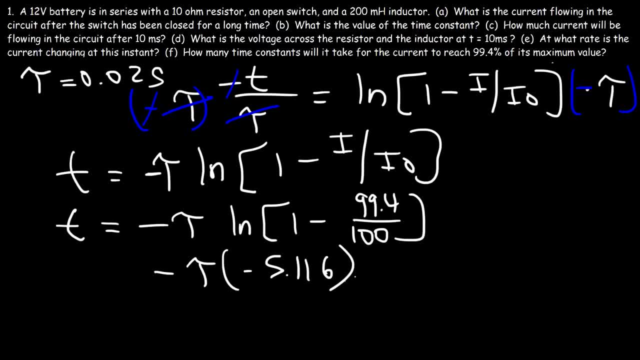 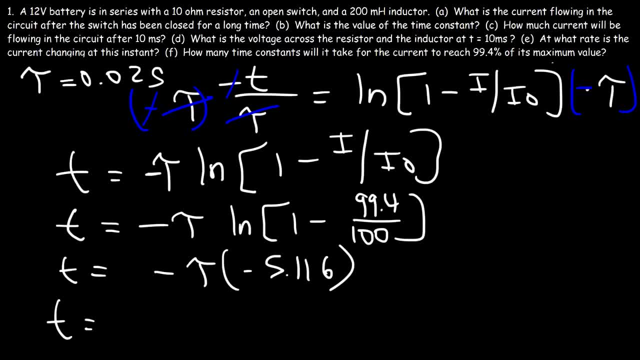 so the two negative signs will cancel, and so it's going to take about 5.116 time constants for the current to reach 99.4% of its maximum value. so this is the answer now. if you need to get the time in seconds, simply replace tau with 0.02. 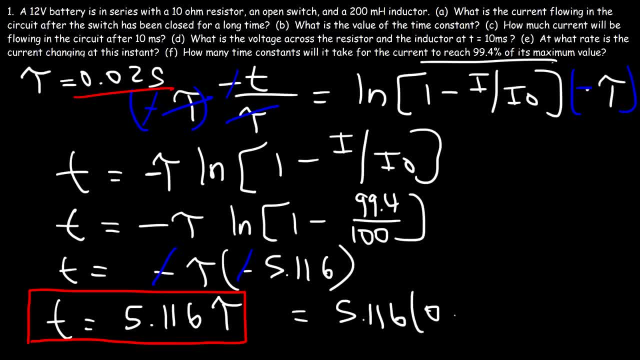 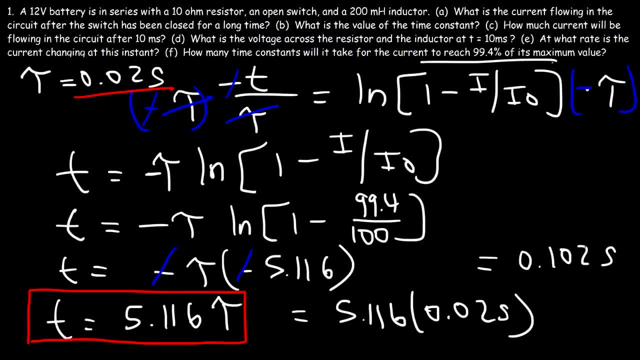 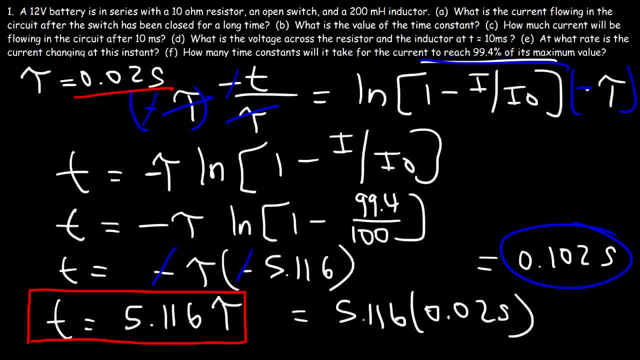 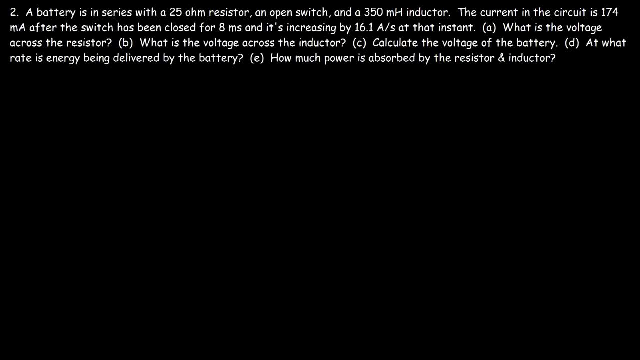 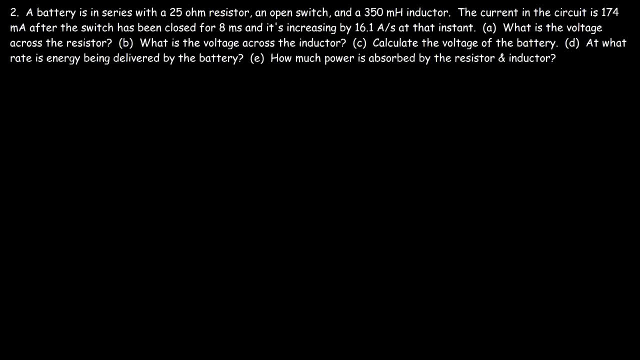 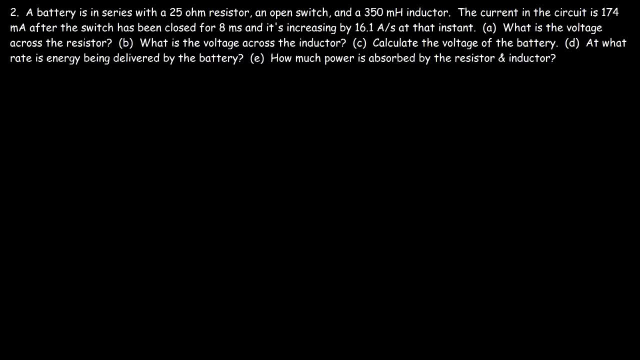 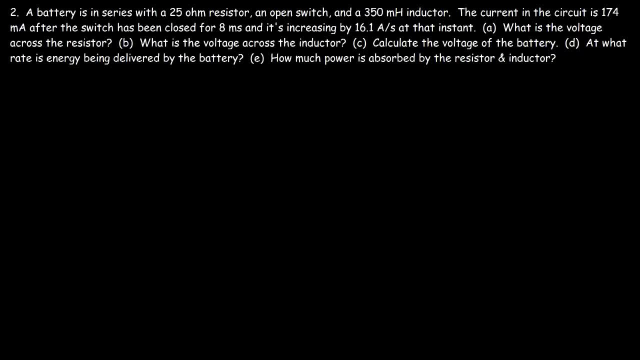 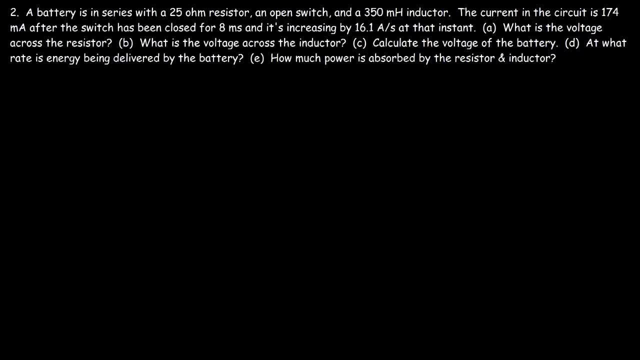 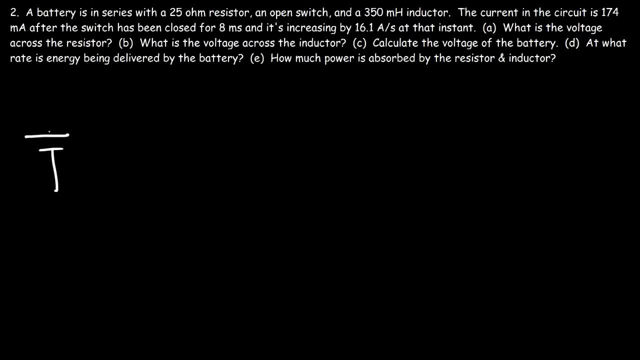 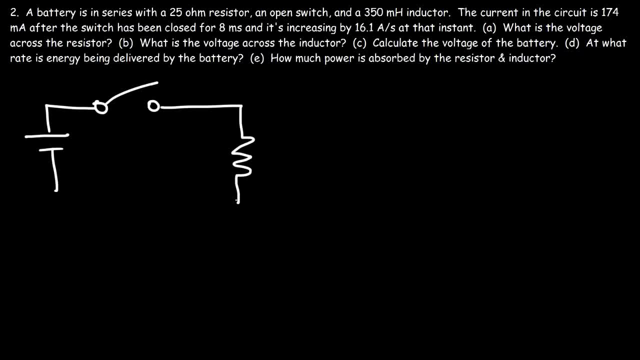 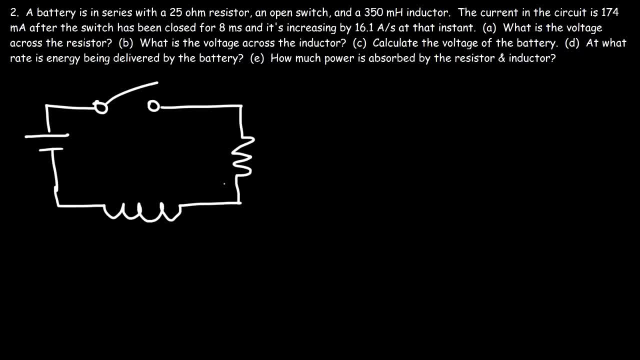 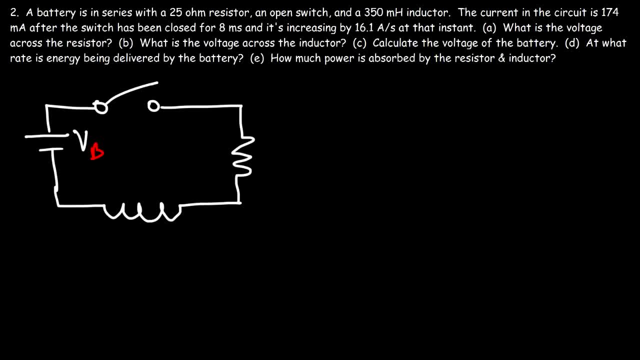 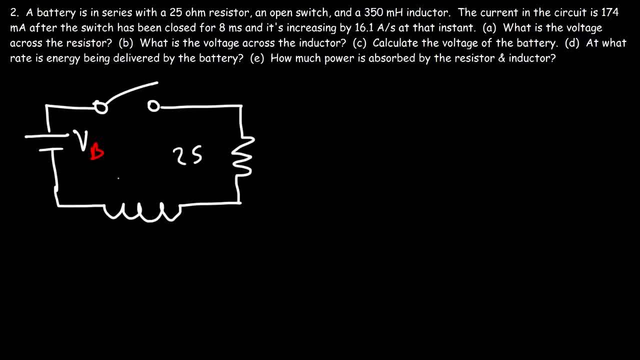 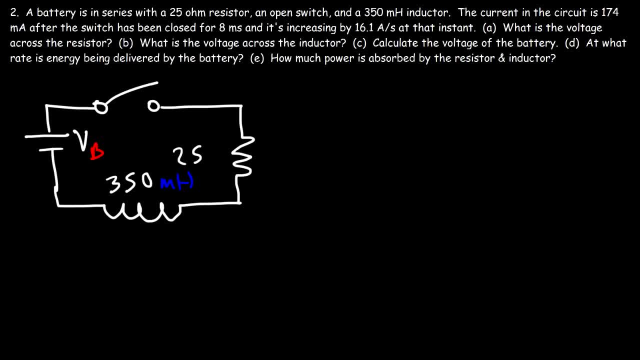 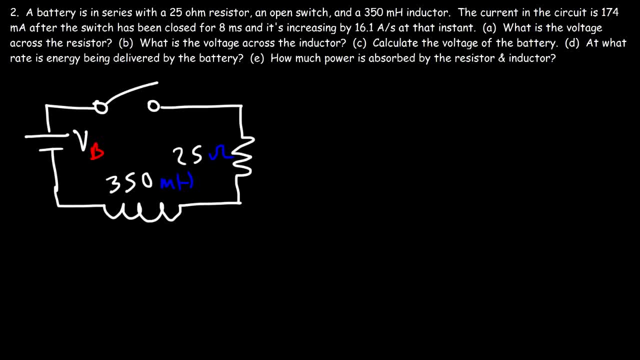 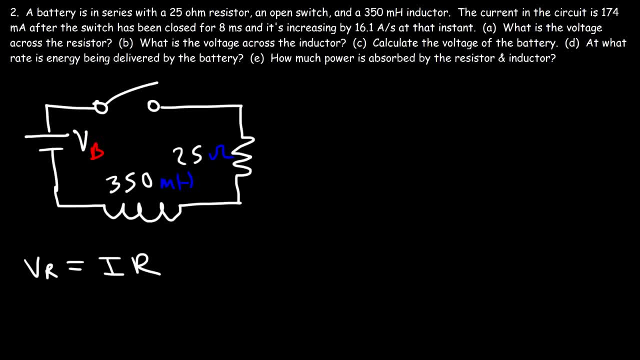 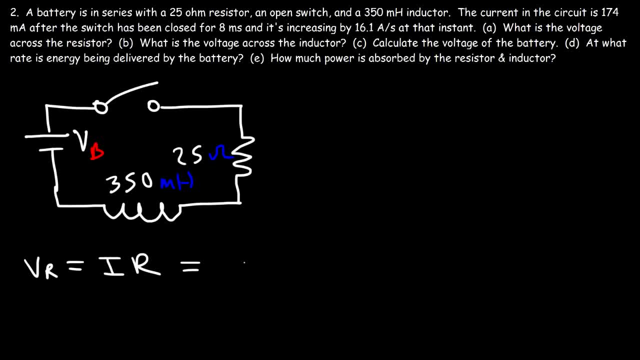 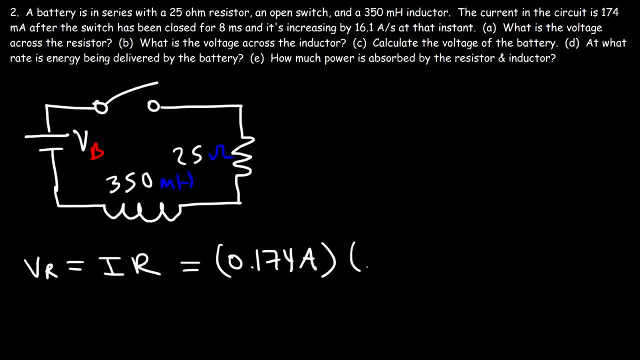 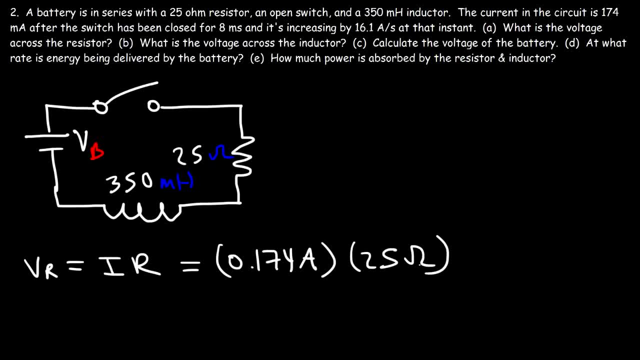 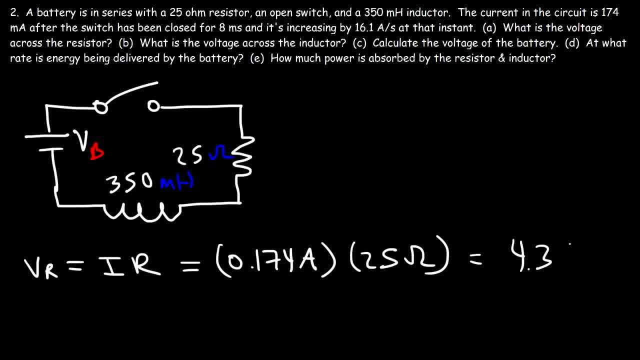 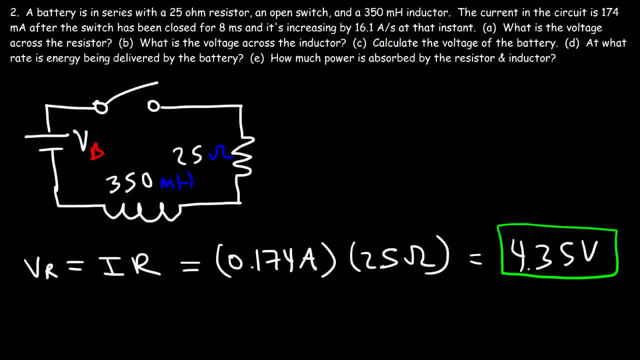 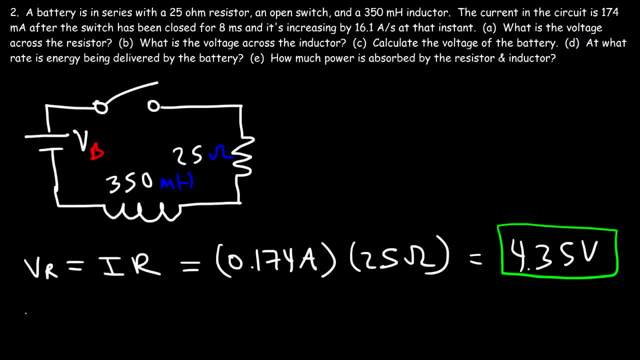 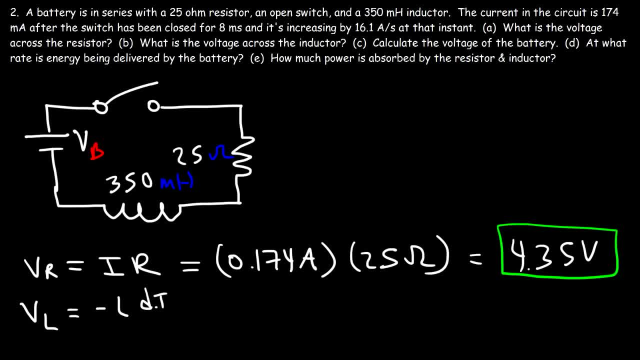 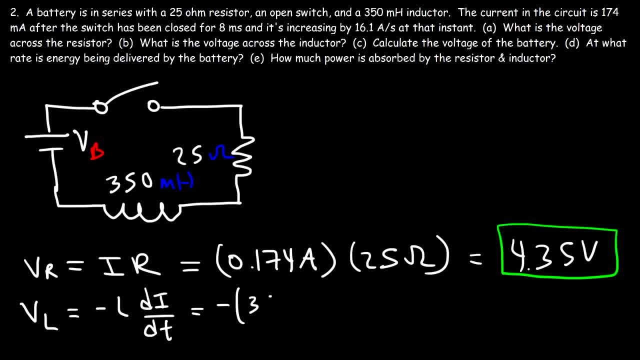 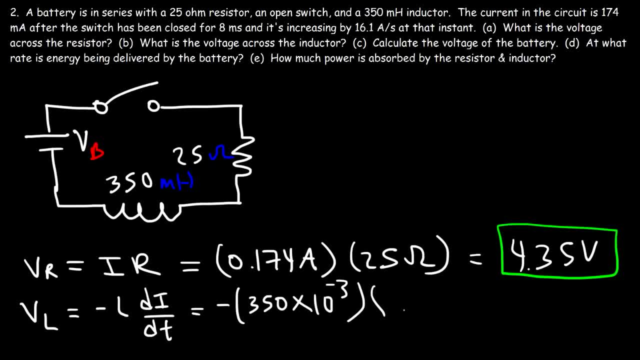 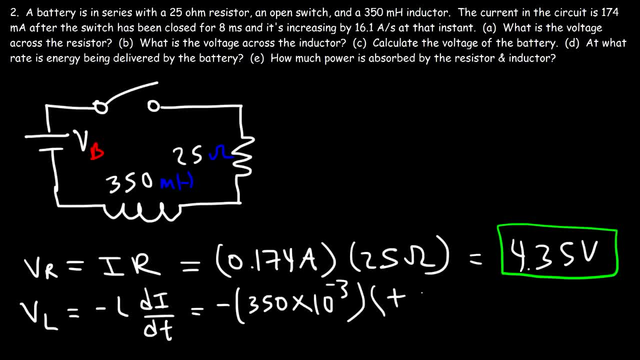 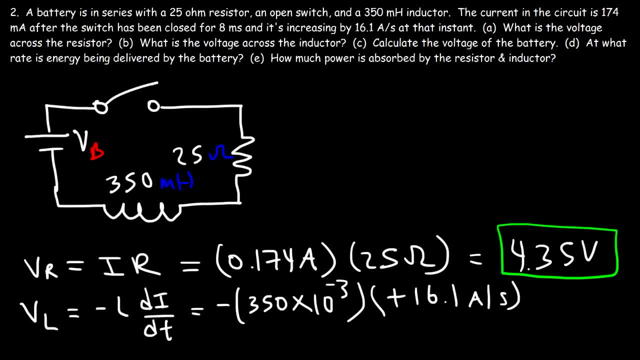 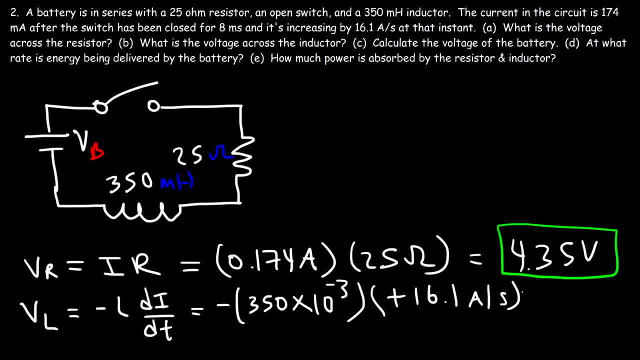 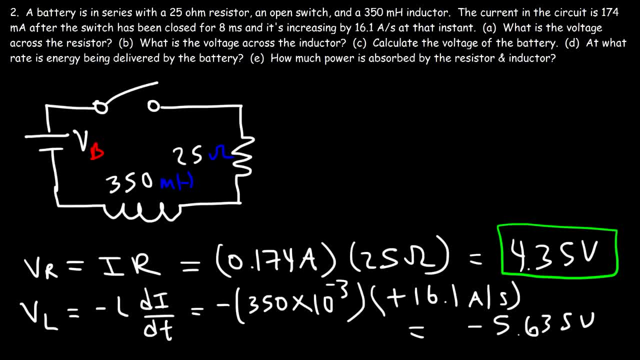 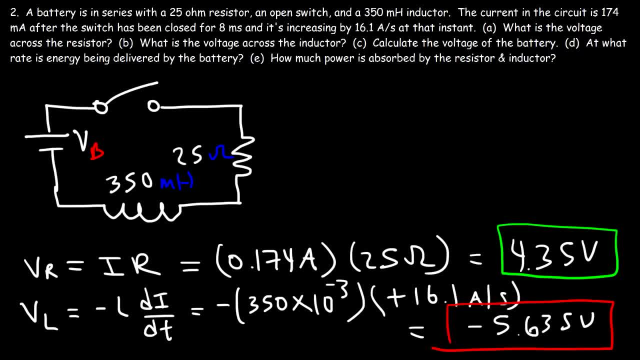 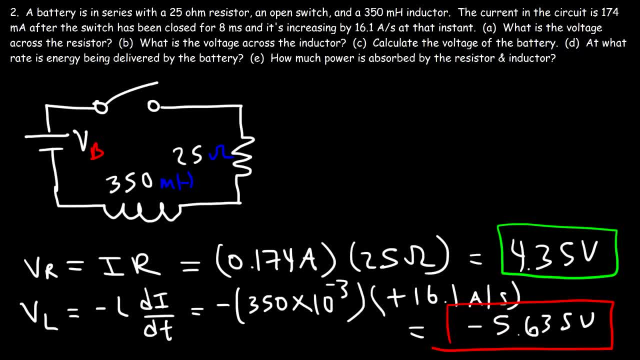 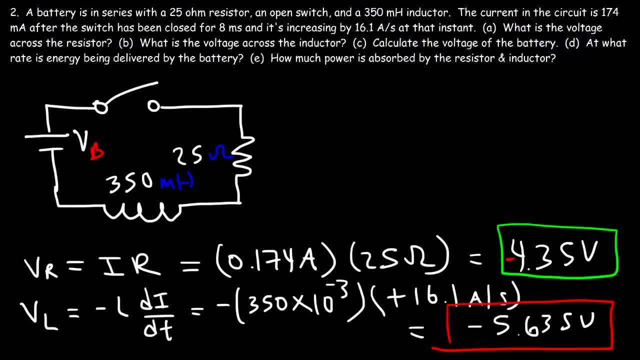 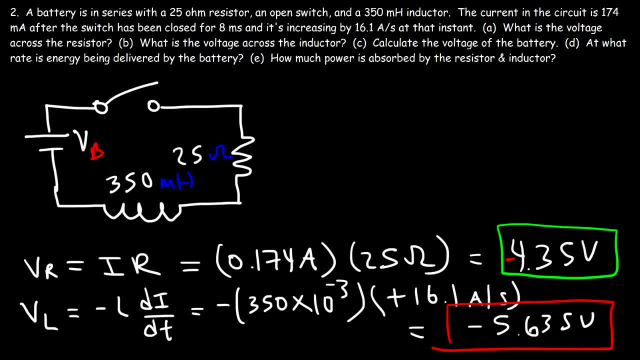 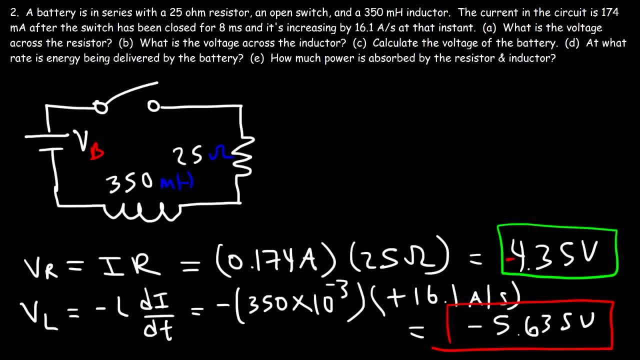 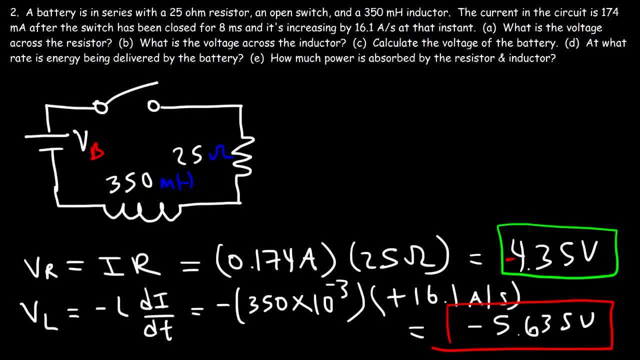 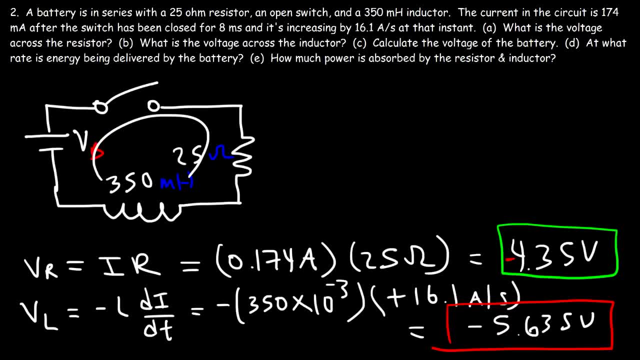 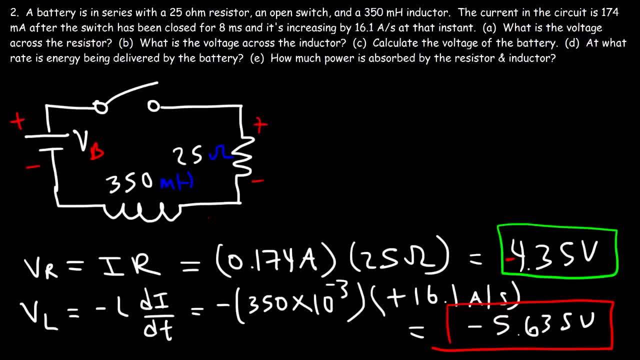 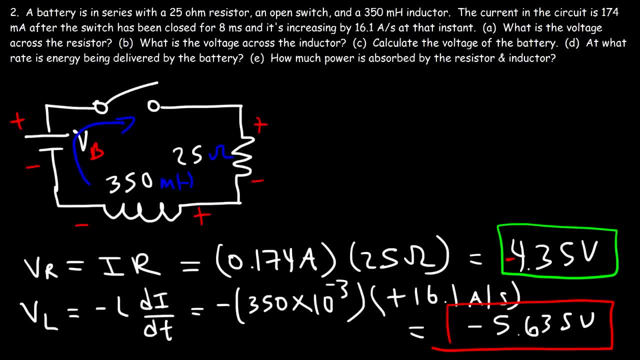 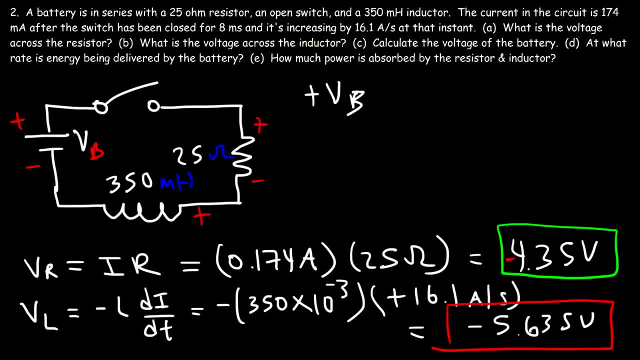 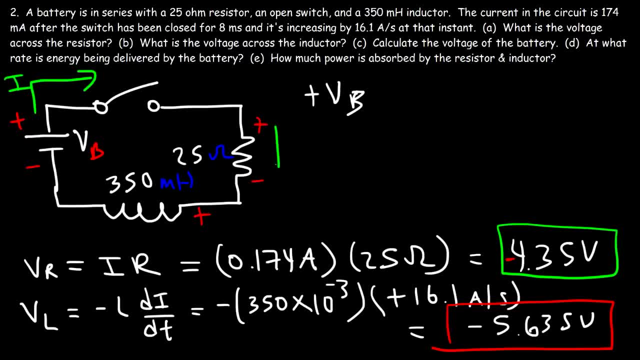 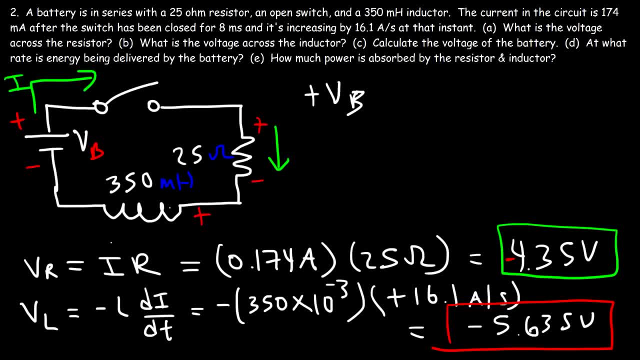 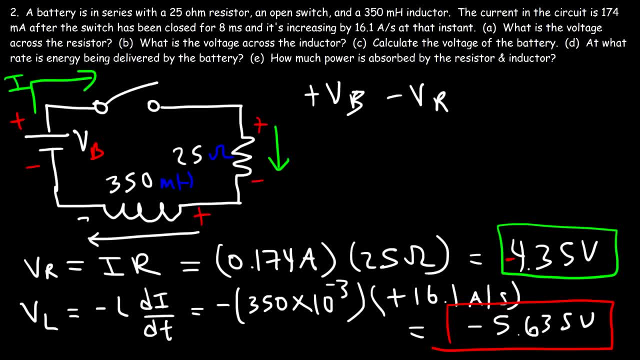 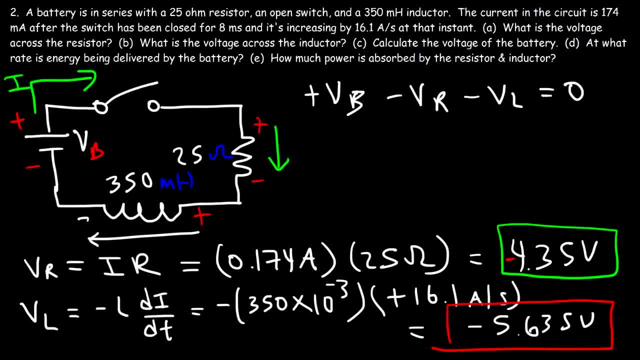 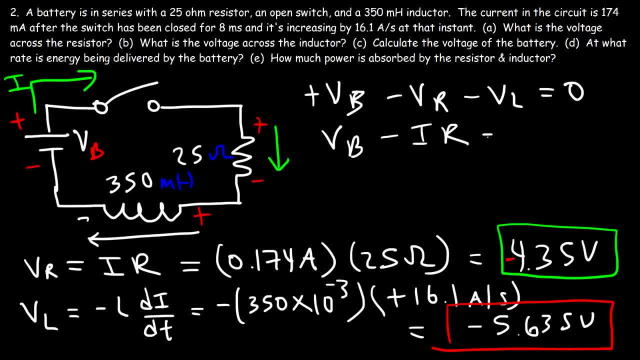 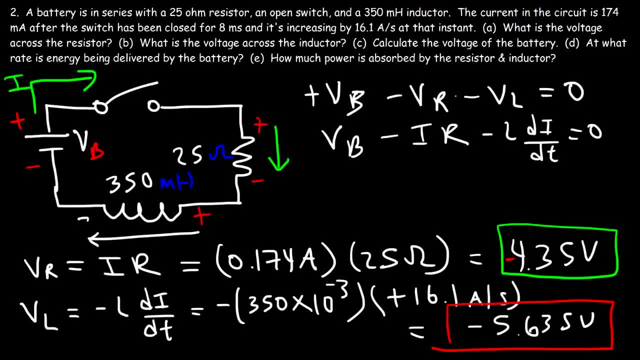 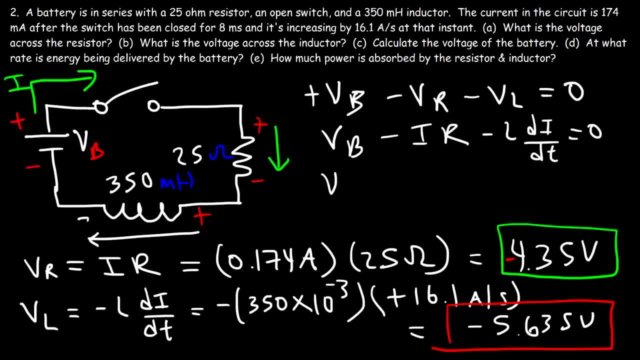 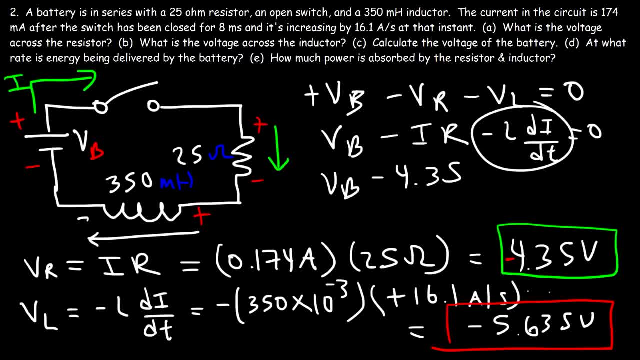 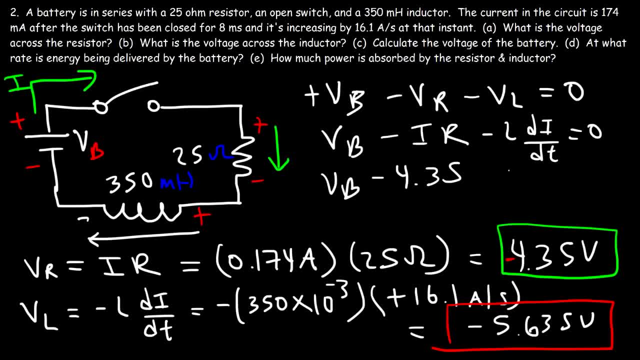 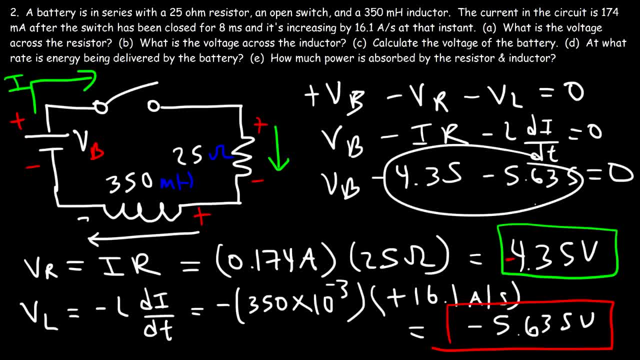 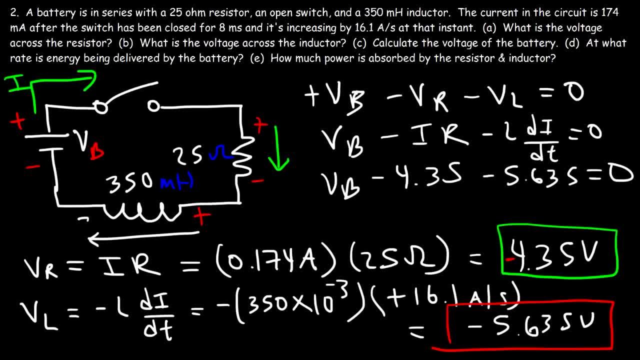 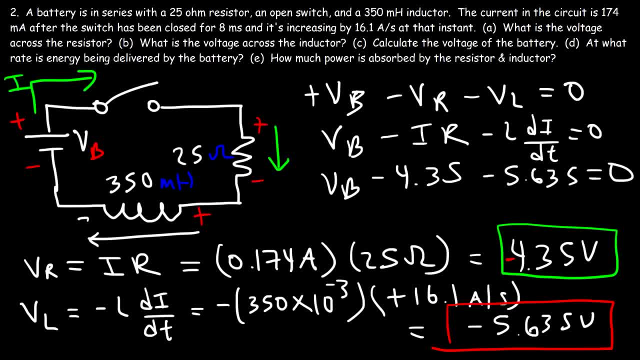 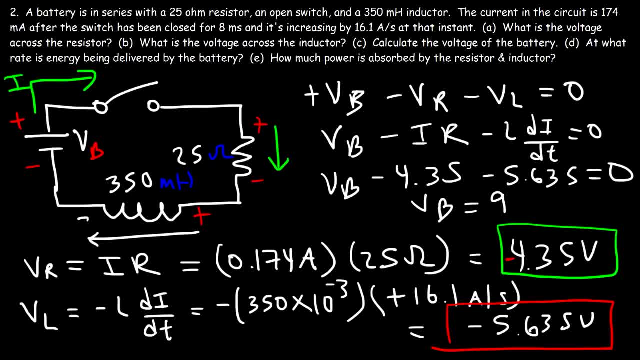 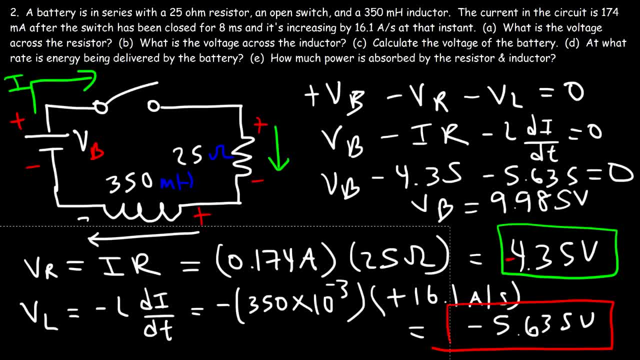 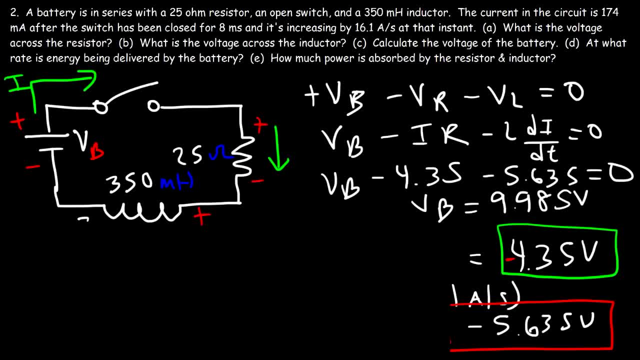 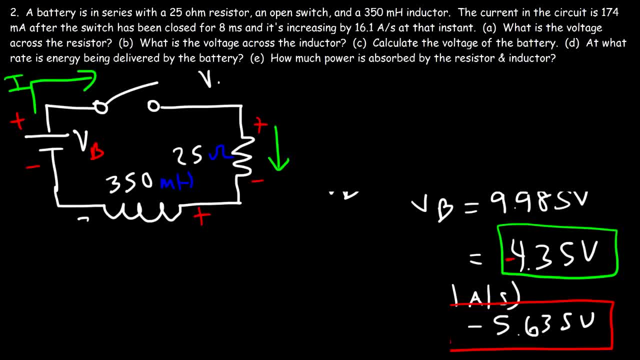 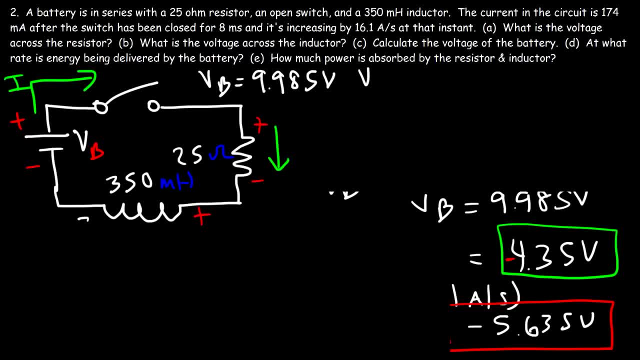 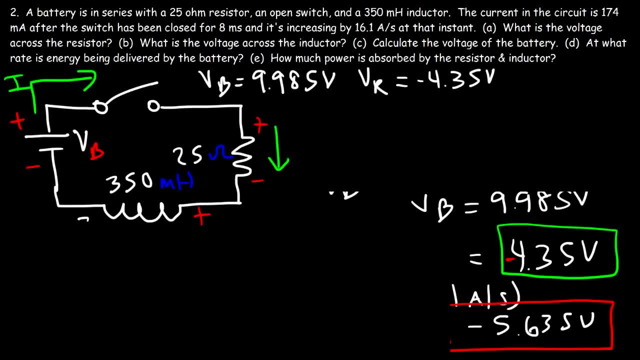 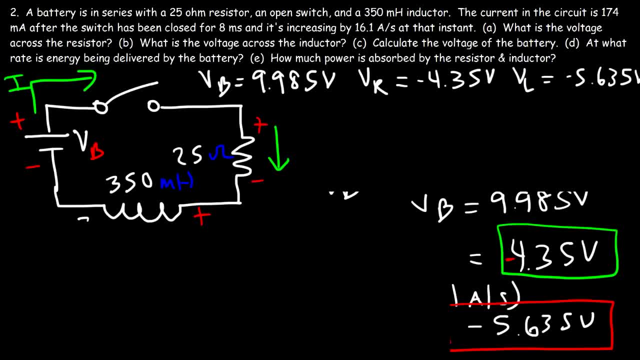 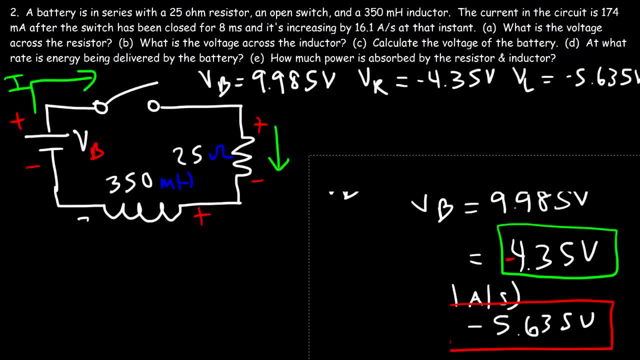 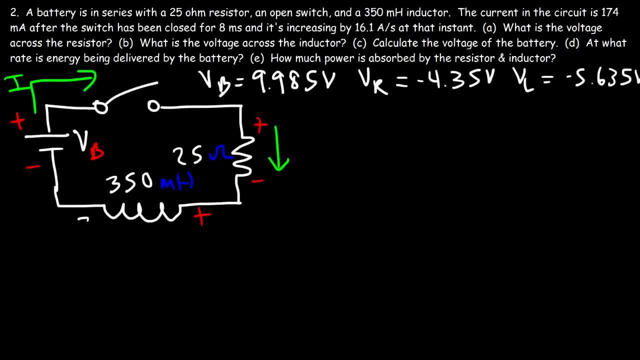 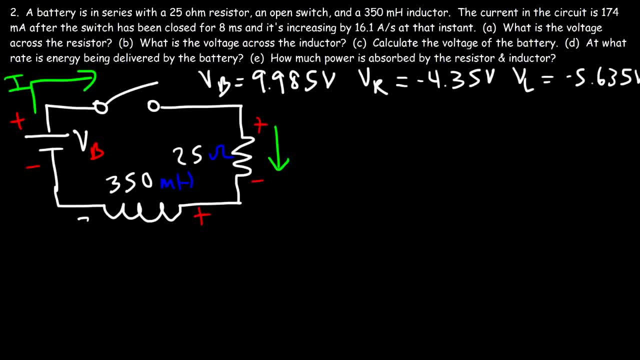 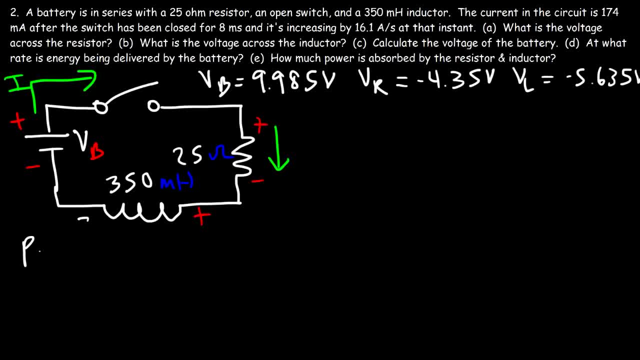 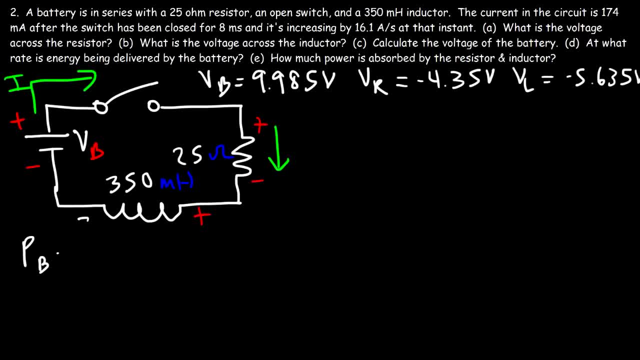 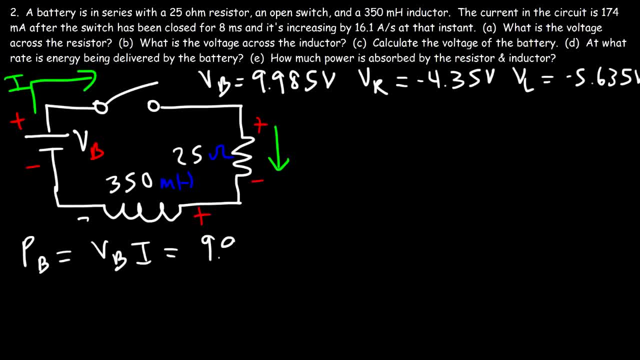 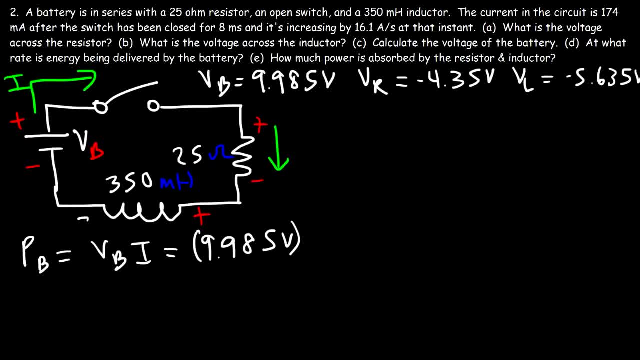 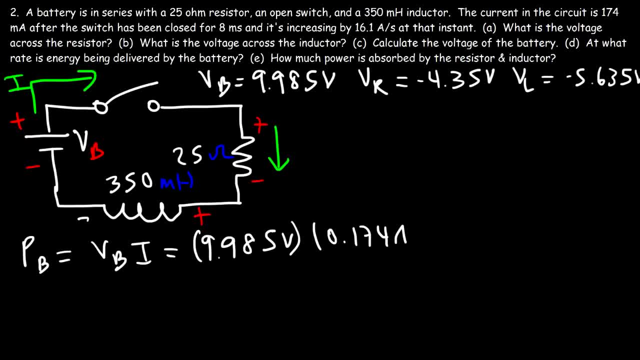 The current is 0.174 amps or 174 milliamps, So this is 1.737 watts. Now, because the battery is delivering energy to the circuit, I'm going to define the system as the circuit. So this system is gaining energy, so we're going to assign this a positive value. 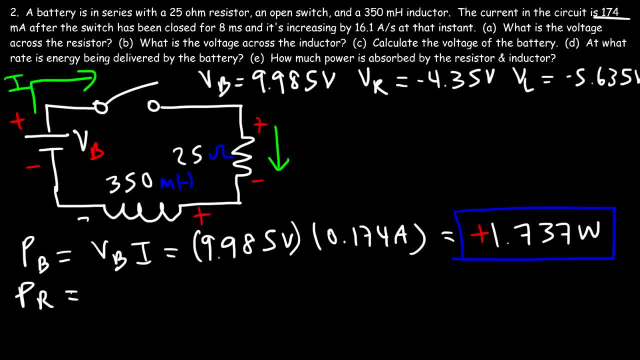 Now, the resistor consumes energy, so I'm going to assign a negative value for that, And so it's equal to: I squared R, That's the power absorbed by the resistor. So the current is 0.174 amps. we need to square that and the resistance is 25 ohms.